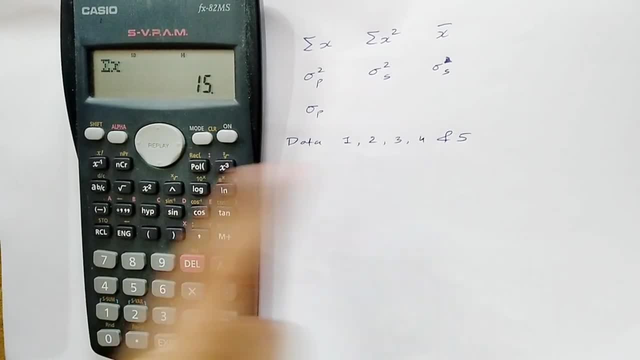 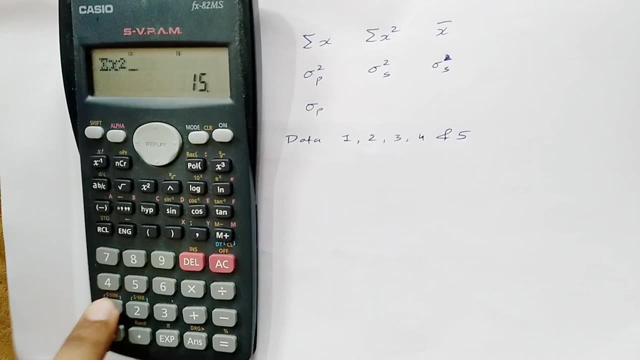 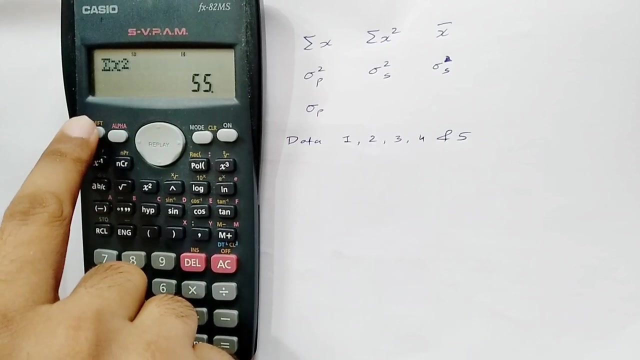 and then equal to That is 15.. So sum of all this value is 15.. Again, press, shift 1.. We want sum of square, So 1 equal to That is 55.. So sum of square of all this value is 55.. Now we want to calculate mean. So again shift, press 2.. 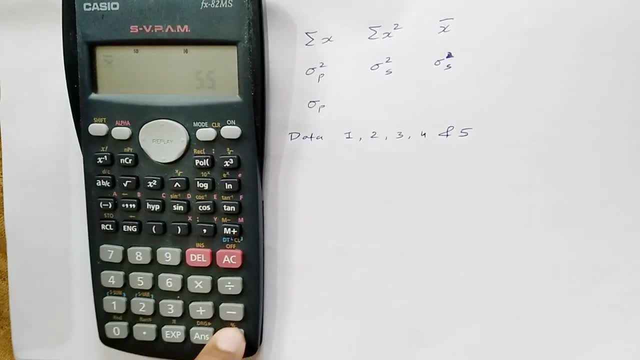 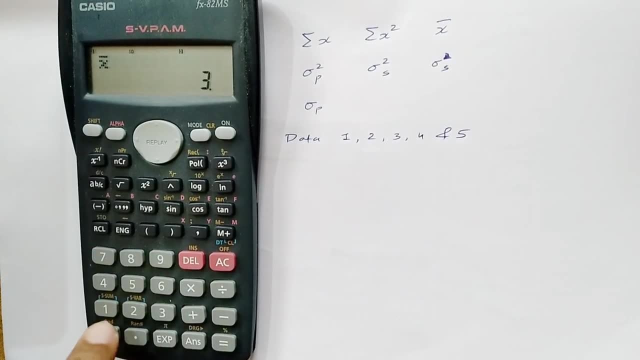 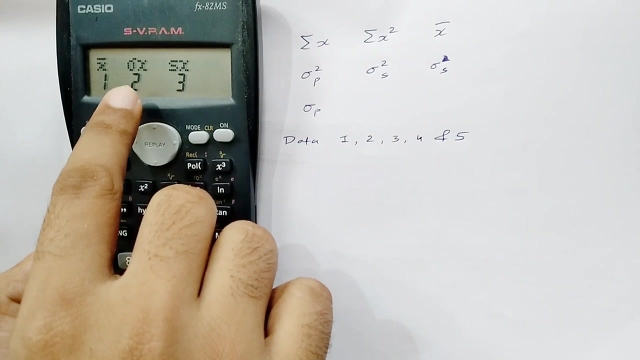 The mean has the first position, So 1 equal to, So the mean is 3.. Now we want to calculate the sum of square, So shift and then press 2.. Now here sigma x, That means the standard deviation. 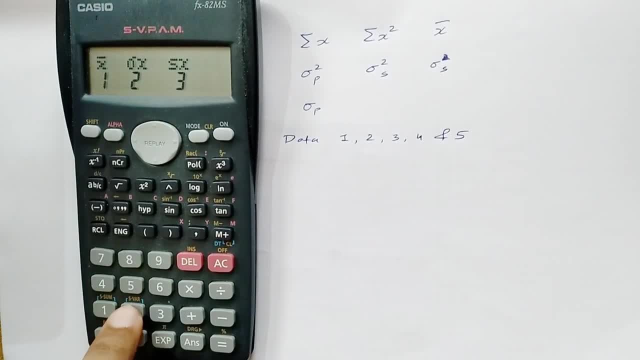 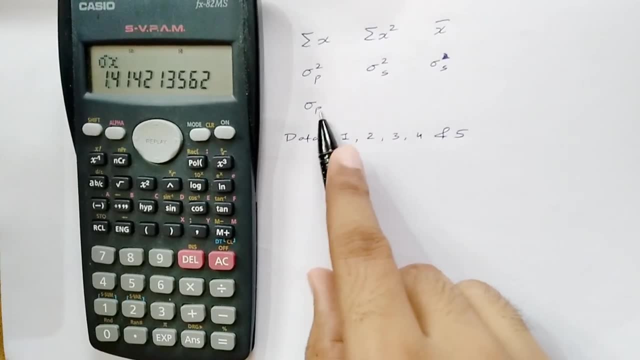 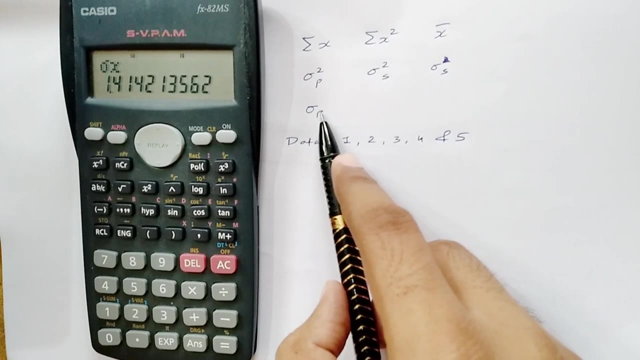 of the population. So we will press 2 and equal to, So that is 1.41.. We get this value, So we get the standard deviation of the population. Also, we want the variance of the population, So variance of the. 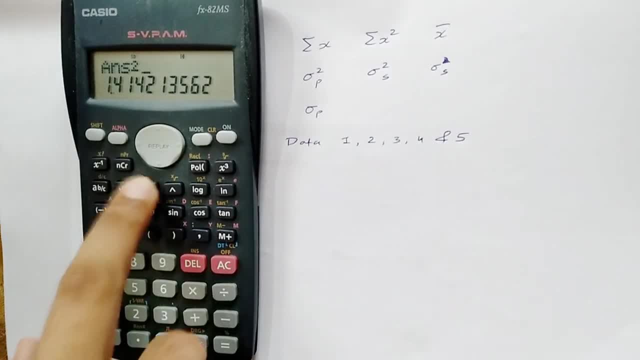 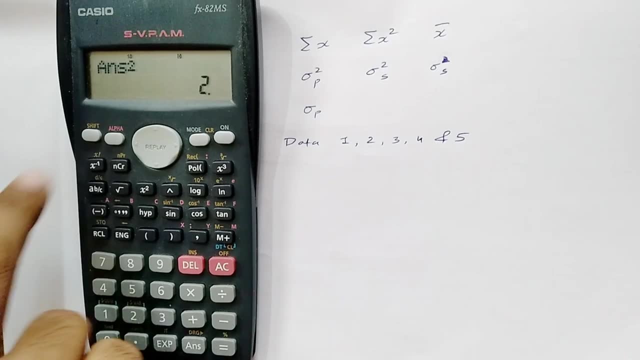 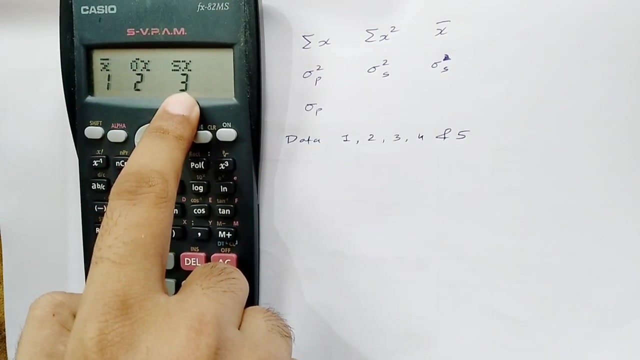 population is square of this value, So square equal to. So we got this value. sigma square p, that is variance of the population. Now we want to calculate the standard deviation of the sample. So shift 2 and then 3.. Here s x, That is the standard deviation of the sample. So press 3, equal to. 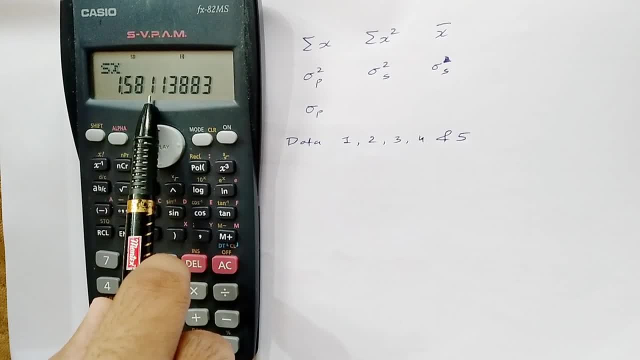 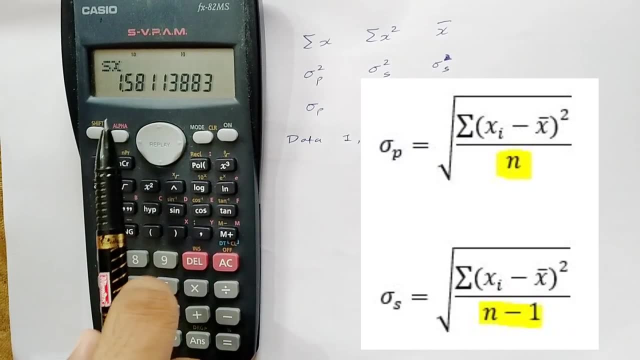 So the standard deviation of the sample is 1.58.. Here there is only change in the formula. in the denominator We have n minus 1 instead of n. So now we want, we get this value, We want the variance. 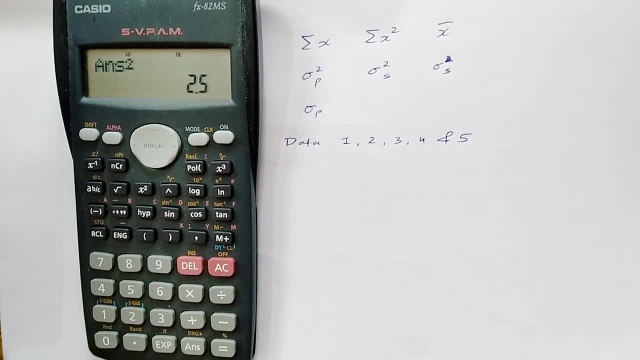 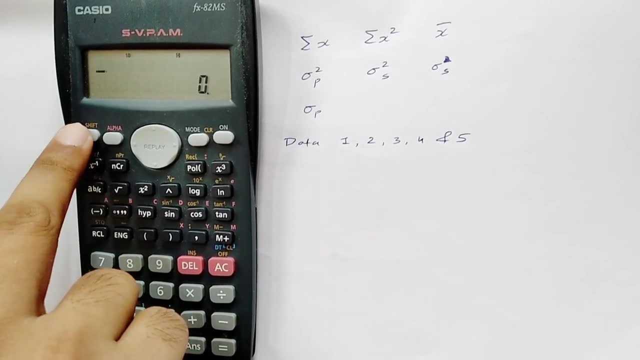 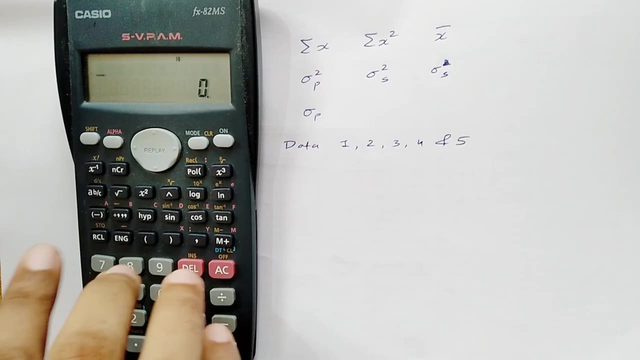 of the sample, So we will square it. Okay, Now our calculation part is done, So again, we follow this routine: Shift clear all equal to equal to. So this will clear all these values Our system will now have if we go for second time. 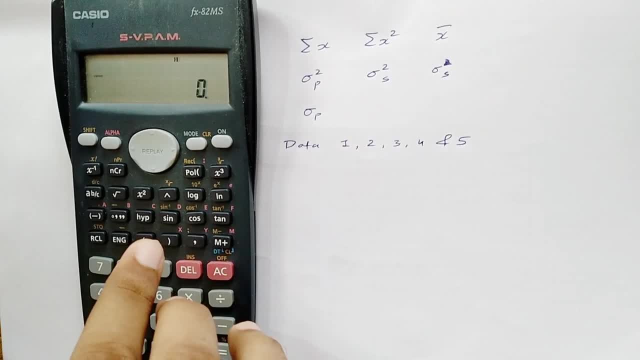 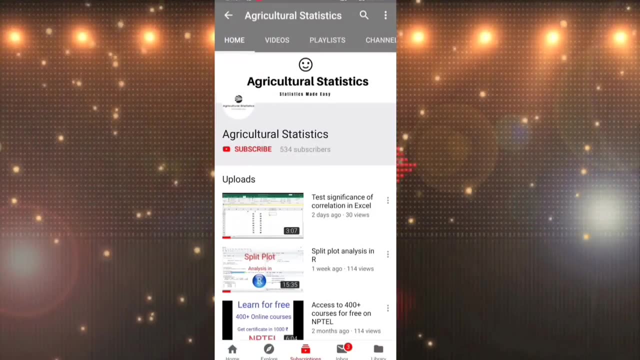 for calculation. it will have the fresh data. So this was all about the calculation by using this calculator. Thanks for watching this video. If you like my work, please do subscribe the channel And click on the bell icon to get the latest notifications.